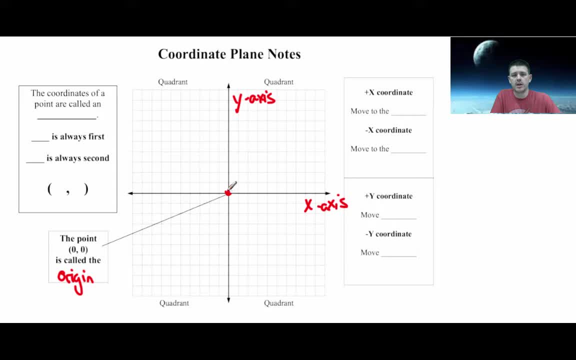 start at that point. anytime you are going to graph your point, Your coordinates- those two numbers that we're going to use to find a point are just directions on how to get there from the origin. The coordinates of the point are called an ordered. 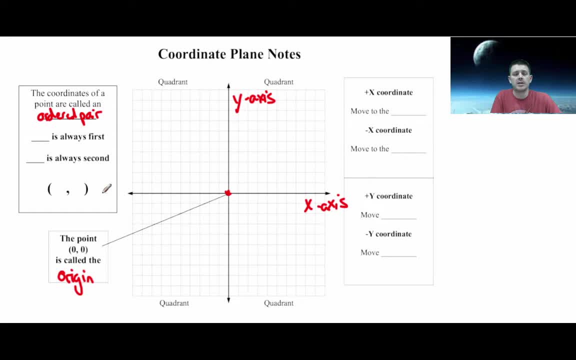 pair. Sorry for my handwriting, I'm going to squeeze it in a little spot. It's a pair of numbers: an x- that's always the first one- and a y, but the order matters because each one tells you where to go along: the x-axis and the y-axis. So you we sometimes see it written as an x and a. 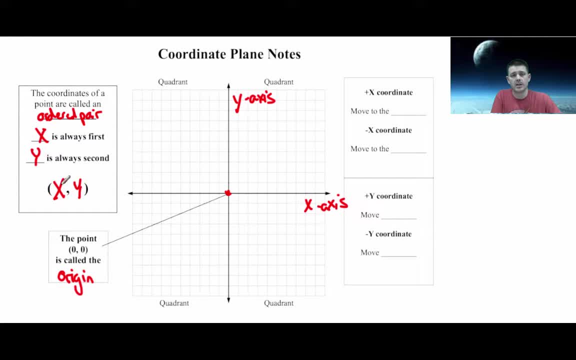 y. Remember. x comes first in the alphabet. X comes first in our coordinates. But basically it's just giving us directions. The first number is the x. It tells us where to go left and right. So a quick way to remember it is: if you have a positive for your x, it means you're going to move. 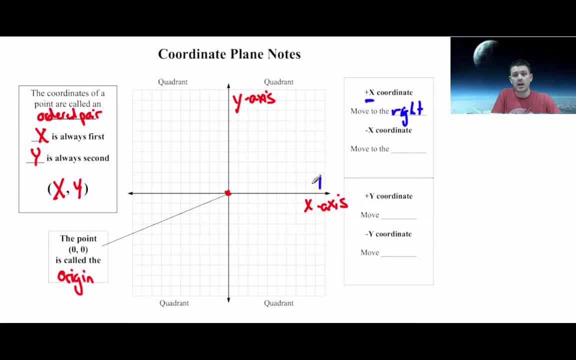 to the right. Because if you think of a number line, as you move to the right on a number line, you move towards the positive numbers Along the x-axis. if you go to the left of 0, you're going to move into the negatives. So if you have a negative x, that means you're going to move to. 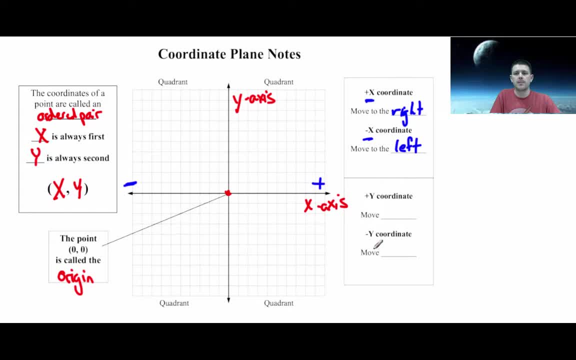 the left, And we'll see some examples of this here in just a minute- Your y-axis, remember that's the one that's going up and down If you have an elevator. as you go up in an elevator, you're counting up in the number of. 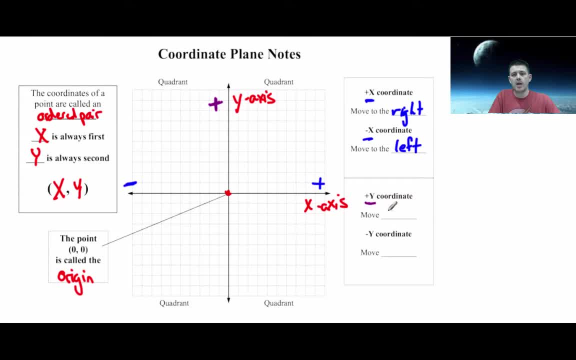 floors 2,, 3,, 4, 5.. So a positive y means you are going up on the coordinate grid, which means if you have a negative y, it means you're counting down the floors, You're heading into the negative. 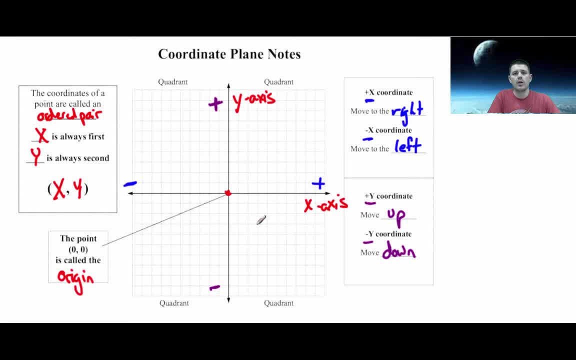 direction. So that gives us a little cheat sheet for us. We're going to practice here in just a second on plotting some points. But there's one more piece that we're missing here and that is the term quadrant. If you notice the two axes, the x and the y, 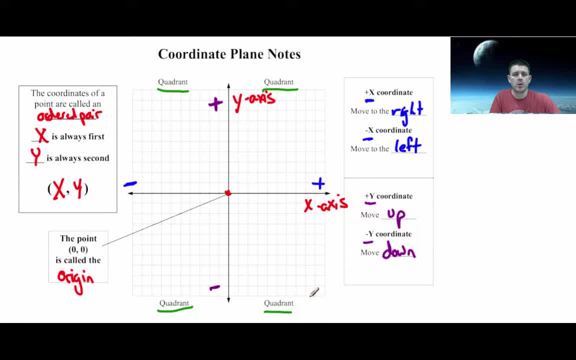 divide the coordinate grid up into four equal parts. We call them quadrants. Each one of them has a name. This first one up here is quadrant 1.. It's written in Roman numerals. This is where the x's are positive and the y's are positive. So positive this direction. positive this direction. 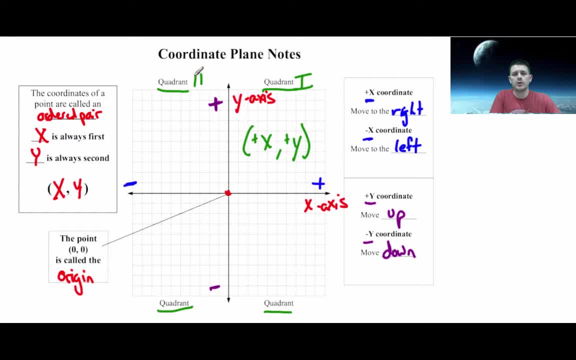 That's what we find in quadrant 1.. Quadrant 2 is over here. Here you went in a negative direction for x, so negative x. but you went up from zero, so that's a positive y. Down here we're going to find quadrant 3.. So you went in the negative x. 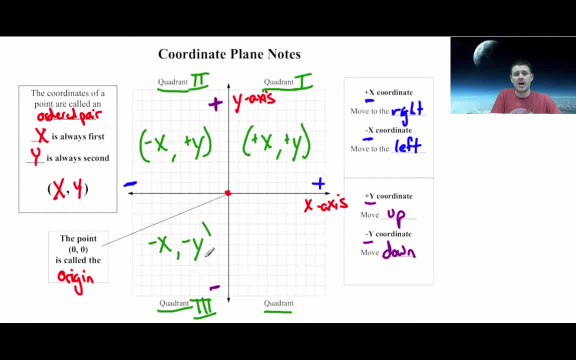 direction. you went to the left, but then you also went down with the y, so that was a negative y. And last is quadrant 4.. IV means one less than V, which stands for 5.. So one less than 5 is 4.. 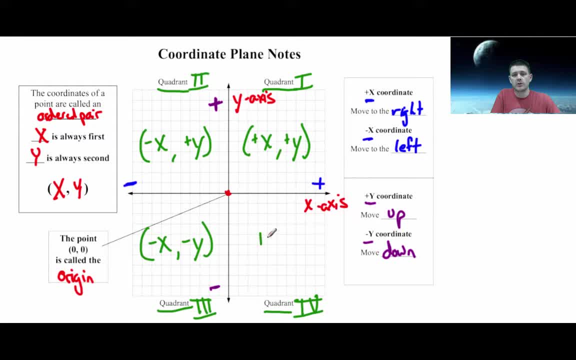 quadrant four. here we went in the positive direction for x, but we went down, so a negative direction for y. Now I know that was a lot of information. feel free to watch it again if you need to. One other note for us is sometimes it's hard to remember the order of our quadrants. 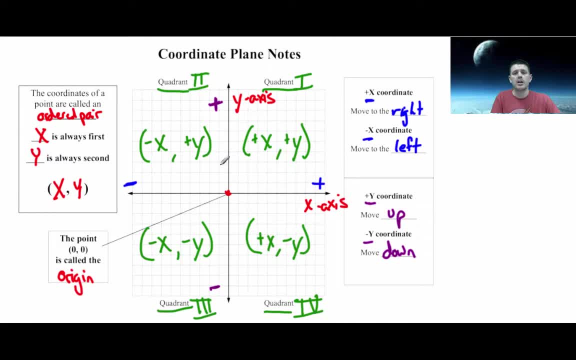 because they kind of go backwards, as we're kind of going around. so I think of it, as we're graphing coordinates, so I think of the c in coordinates. picture how you would draw a c: you'd start up here, you'd wrap around and end up down here. one, two, three, four. that's the order that our 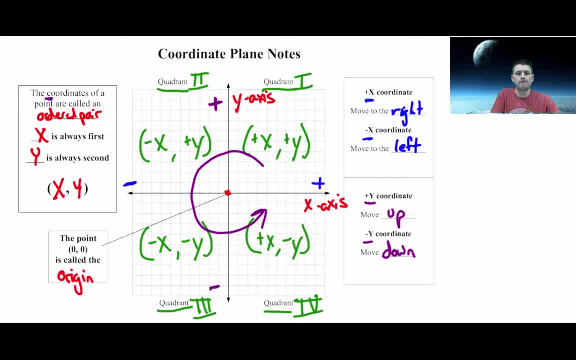 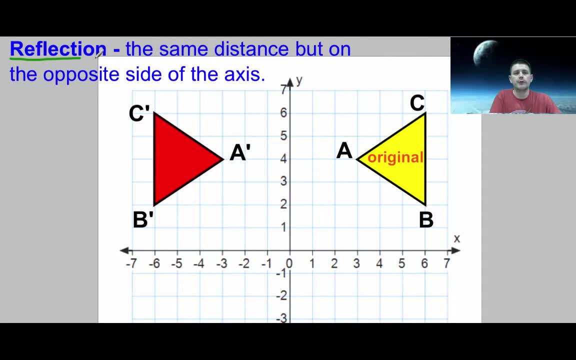 quadrants are numbered. So what we're going to be talking about for the next part is what it means to reflect a shape. so think of reflections in a mirror. it's kind of a another copy of you as you look in the mirror, but it's on the other side of the mirror. it looks like it's in another room, on. 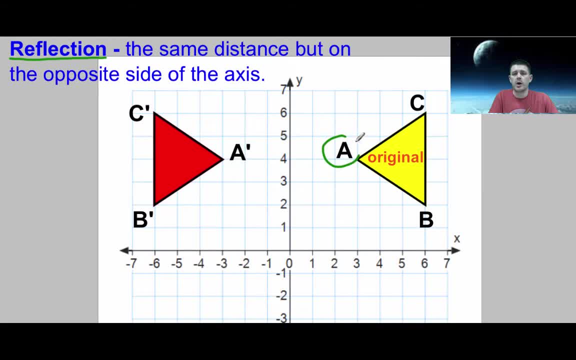 the other side. Whenever we plot a point, we always name it with its name or with its coordinates. when we reflect it, we're going to notice the reflection or the new version by that little tick mark next to it. we call would call this point a prime. it's the new version of point a. 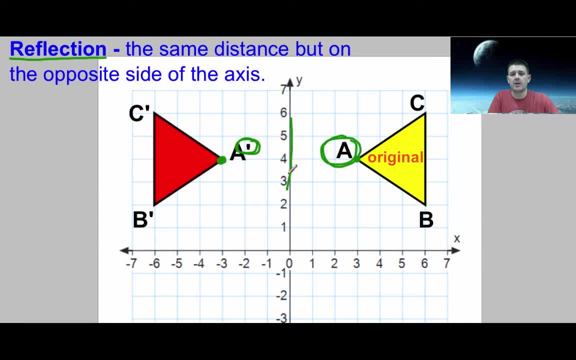 after it's been moved, but basically think of reflecting as kind of folding over one of the axes, in this case the y-axis. we took that shape, the yellow one on the right, and we kind of folded it over, almost like we folded it over, and we're going to be able to see the reflection of the. 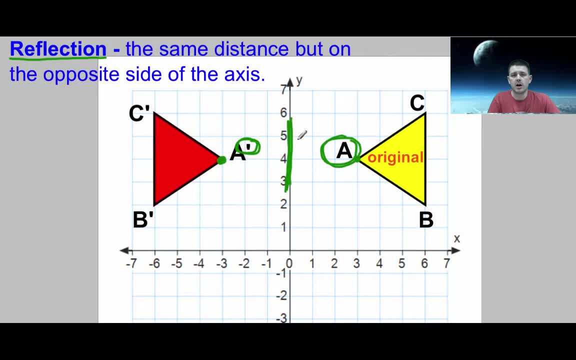 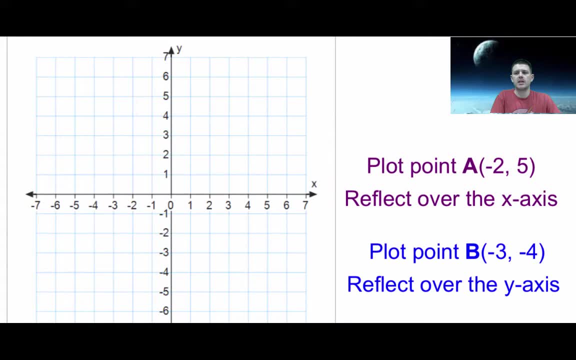 whole of the page in half. the reflection is what we would get on the other side and we're going to see that here for an example for us. So we get this. one says: let's pick our purple here. it says the plot point a at the point. 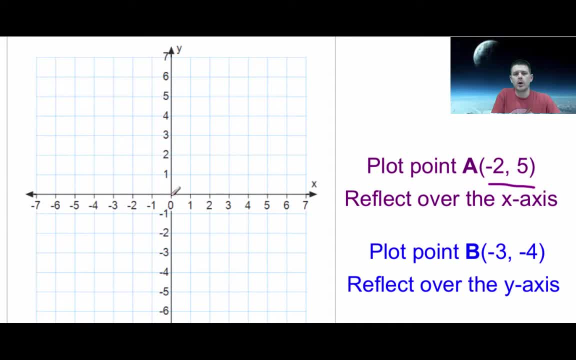 negative 2, 5.. So remember your, your coordinates are always starting at 0 negative 2. that's my x. so remember, the first number always tells you left, alright. so I'm going to go left to negative two. my second coordinate is negative zero. it's negative six. Longer it goes from the same. one right, so I'm gonna go left to negative two. my second coordinate is negative, one blue. So that's what we have: to limit the eliminates model, that personality function class. number three is important, and we're going to bebad that when we have the coordai Б' in every Fasciano variable. So what we're meant to do is to evaluate all class. 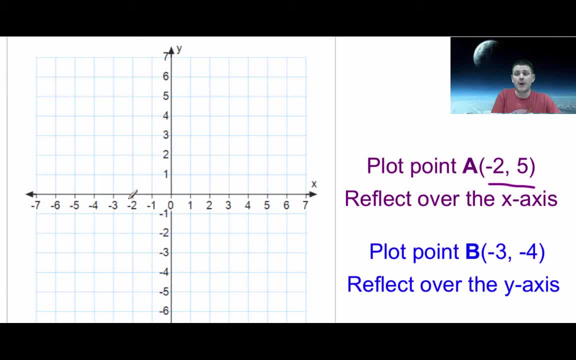 negative two. my second coordinate was five, that's for y, that's a positive five. so that means i'm going to go up five and that's my point a. always make sure you name your point or label it so we know which one you're talking about. now it says we're going to reflect over the x axis, basically. 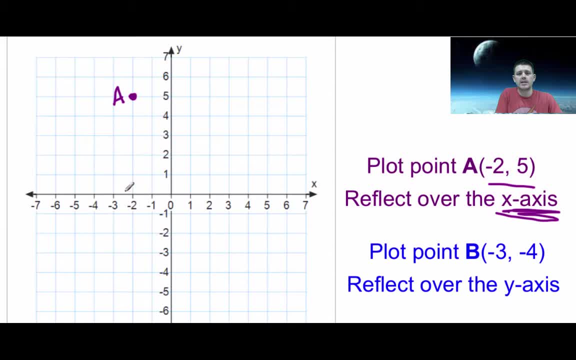 we're going to fold it over the x-axis. remember our x-axis is this one down here running across the page. so what's really going to happen is we're going to fold the top down to the bottom. so the easiest way to think of it is it's just going to go in the exact opposite direction. 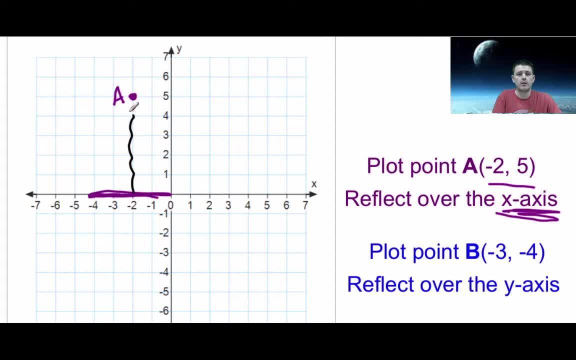 from the bottom. i went up: one, two, three, four, five units up. so i'm going to go straight down: one, two, three, four, five units straight down. that's the reflection of point, a same distance from the line, but in the opposite direction. i just went to the opposite side of the 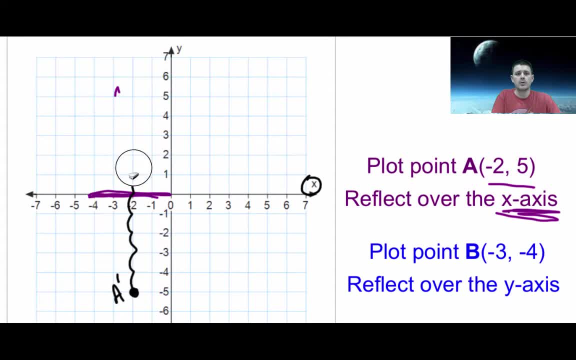 x-axis. i'm going to get rid of a little bit of that. didn't mean to get rid of point a here, but now we're going to try it again with point b. again, it's just plotting your point and then reflecting it over one of the axes, so point b is at negative three, negative four. 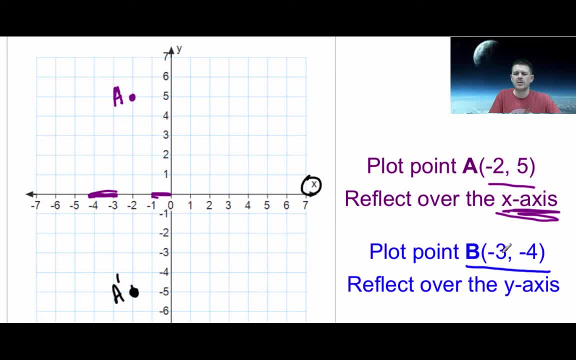 so first number always tells you left or right. as somebody said in class, you got to walk over to the elevator so you got to walk along the ground before you can take an elevator up or down. so start at the zero. we're going to go left to negative three, one, two, three and then we 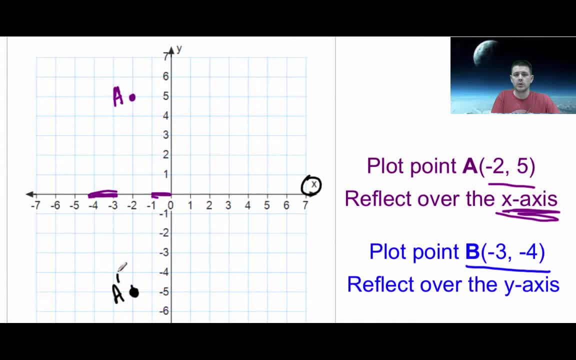 want to go down to negative four: one, two, three, four. so here's point b. this time we want to reflect over the y-axis, so you got to find the y-axis. i like to kind of highlight it or make it stand out. but here's my y-axis, the one going up and down. so really just think of it as b is to the. 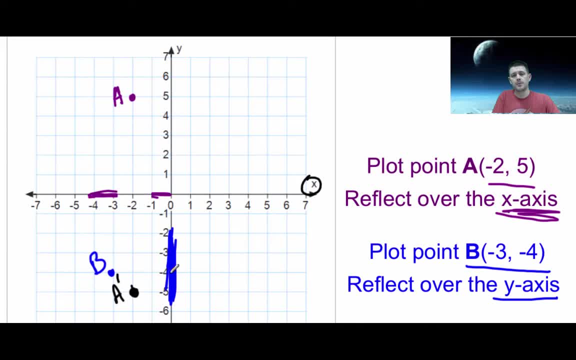 of this y-axis so I want to map it over to the right. It's one, two, three units to the left, so I want to go one, two, three units to the right. I just want to go in the opposite direction across the y-axis when I reflect it. So B was at the point. 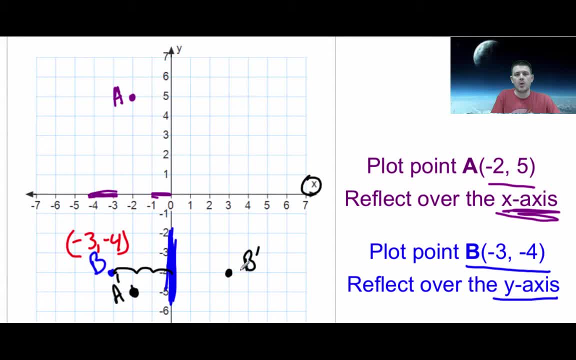 negative three, negative four. When we go to the new version, you'll notice, this time we went to the right, one, two, three, so a positive three, but we still went down four, so still a negative four. So notice when we reflect over the y-axis. 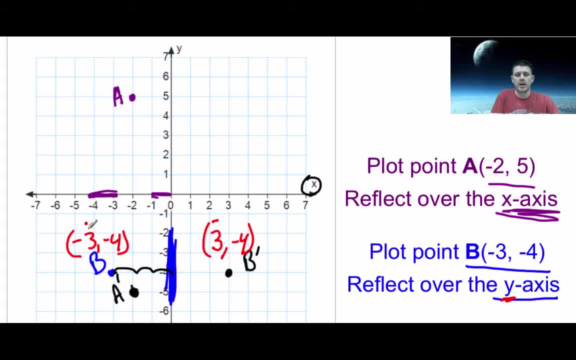 the x is what changed. It went from a negative three originally to a positive three now. It flipped to the other side of the y-axis. but a reflection is just about finding that axis. what am I folding over or reflecting over and go? 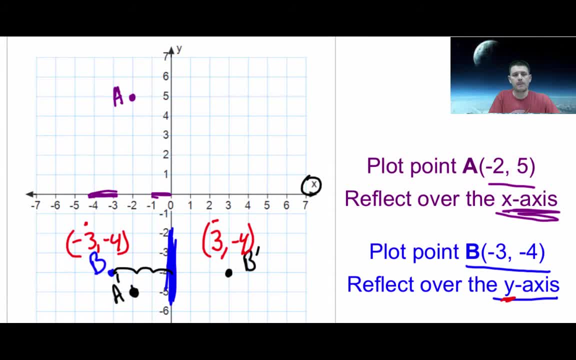 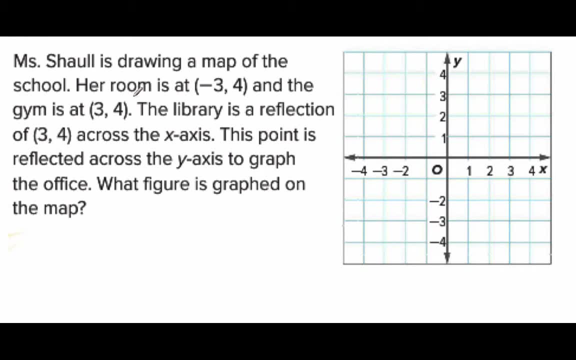 the same units but in the opposite direction. So let's see another example here, quick. It says Ms Shawl is drawing a map of her school. Her room is at negative three, four. So let's find that one Negative three. that's my x, That's always my left or right. so I'm going to go one, two, three. 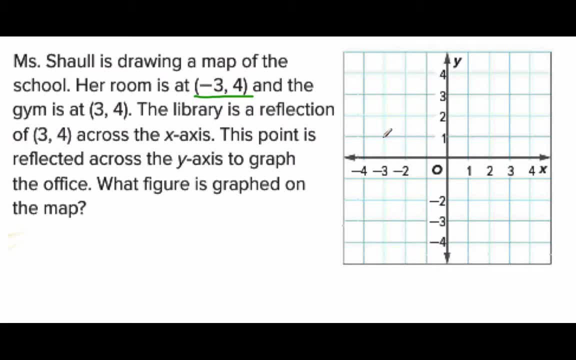 to the left, and then a positive four. for y means I go up one, two, three, four. I'm going to call this. the classroom, That's her room, And the gym is at three, four. So first number is the x. so that's going to tell. 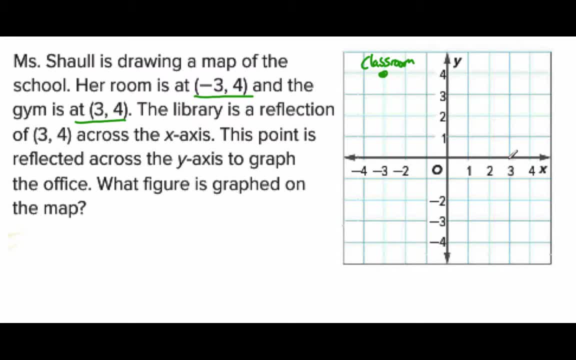 me left or right. a positive three means go to the right. three positive four means go up four. and here is the gym for her particular school. It says the library is a reflection of point three, four across the x-axis. So here is our point. 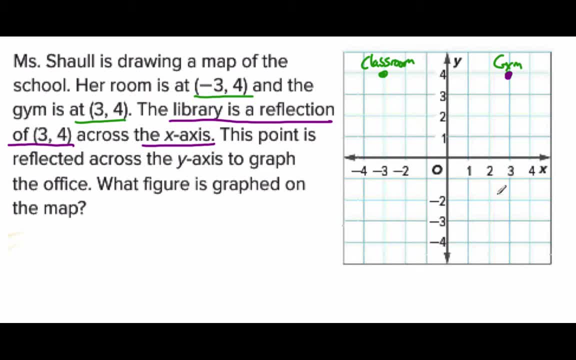 three, four. up here the gym. We want to reflect it over the x-axis, So look for the little x down there. That means we want to fold over this line. So all I do is I just figure out, I'm up one, two, three, four units up. So I want to go one, two, three, four. 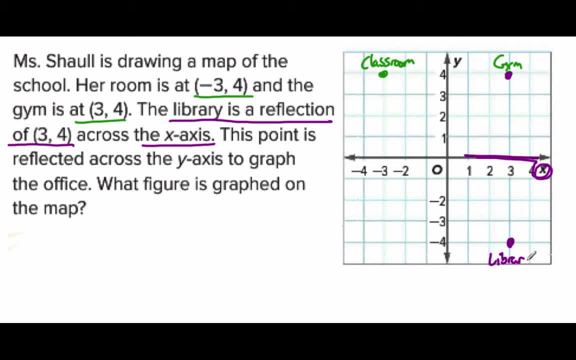 units down And this is my library. Now it says this new point is reflected across the y-axis in order to find the office. So my new point here: for the library, I want to reflect over the y-axis, which is the one that runs up and down. So I just want to go from one side to the other. 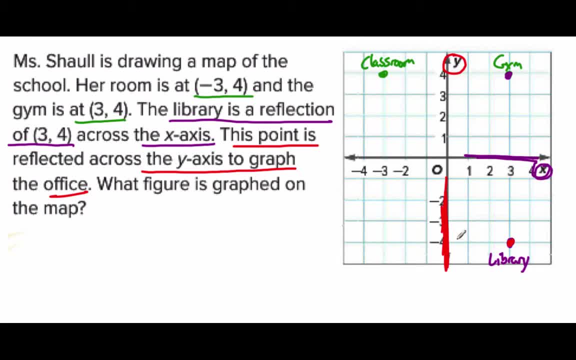 Here I was one, two, three units to the right, So I want to go one, two, three units to the left. This is going to be my office- Then, if we were to, If we were to connect these points- I know it doesn't say that, but I know one of our next problems- 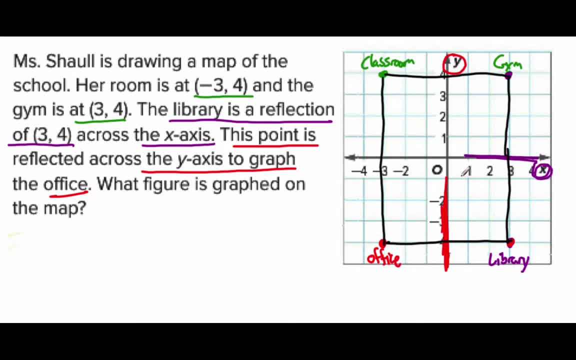 is going to have something similar. We can connect those points and you notice that it makes a rectangle And then we could very easily count how many spaces are each of the different classes or different rooms away from each other. But by plotting those points we can actually create. 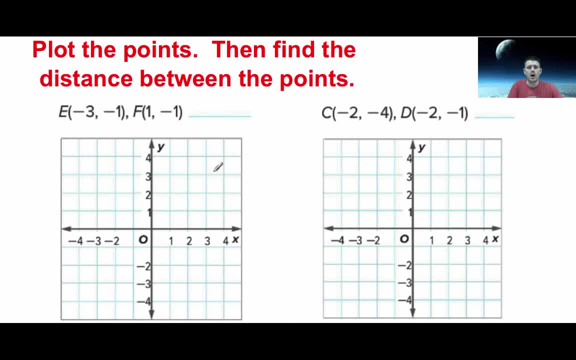 some shapes that go with it. All right, last little bit: finding distance on our coordinate plane. So if we were to connect these points, we could very easily count how many spaces are each of the. Now we want to find out how far is it between two points. The easiest way to do that is to go ahead. 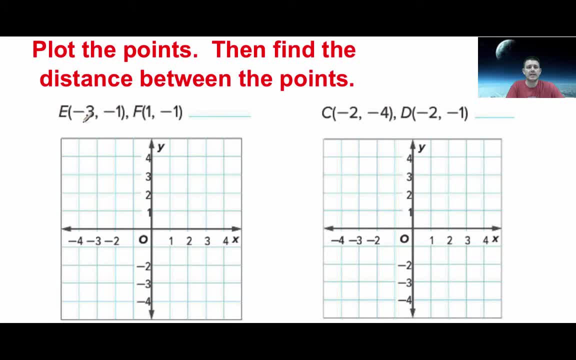 and plot the points and then just count the distance. So point E is at negative three. negative one. Remember first number tells you where to go along the ground. So we want to go left to negative three. And then we want to go down one spot to negative one. 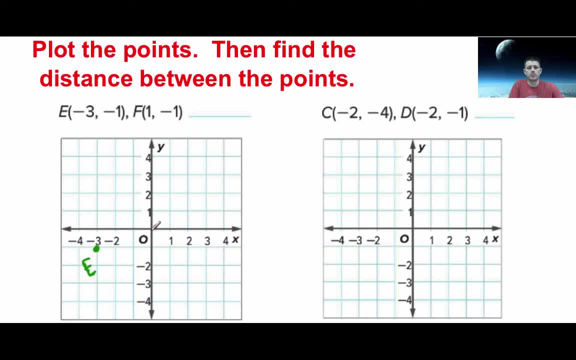 F is going to be at positive one, negative one. So in this case I'm going to go right to positive one and then down to negative one. That's point F, And now we want to find the distance between those points. So we just want to know: how far is it from E to F? Well, it's really just how many. 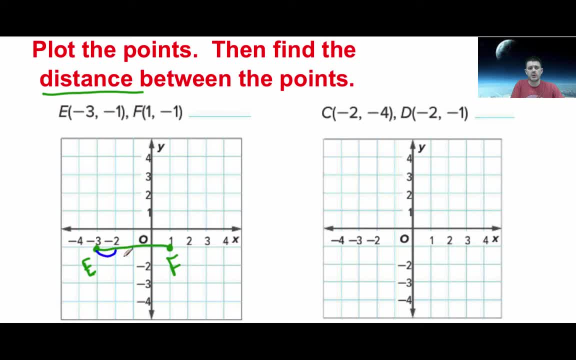 steps. how many hops would it take to get there? So for me it would take one, two, three, four steps to get there. So they are a distance of four units apart. Let's see another one. C is at negative two, negative four. A lot of negatives in these problems, just to get you used to it. 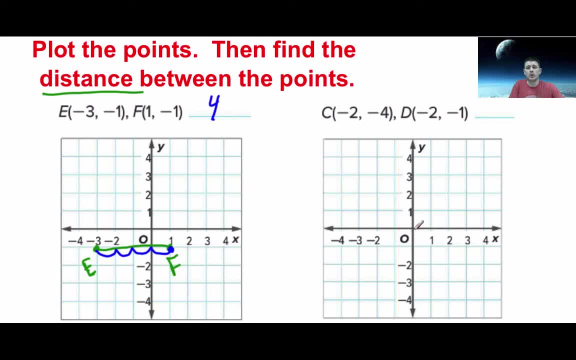 So first number is left and right, So I'm going to go left to negative two. And then the second number is my Y. A negative means going down, So I'm going to go down to negative four, and that's point C. Here D is at negative two, negative one. So first number is left and right, So I'm 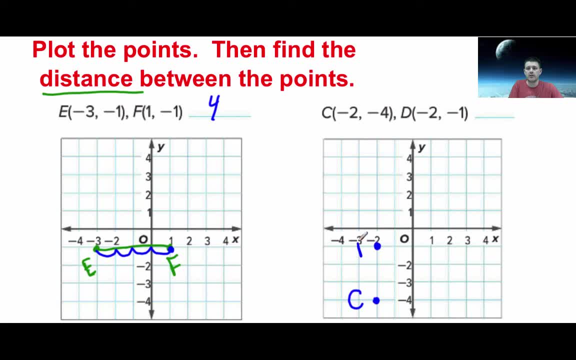 going to go left to negative two and then down to negative one. That's point D. Now I want to find the distance, So I just count: It's one, two- oh, lost my pen there. One, two, three steps, So don't. 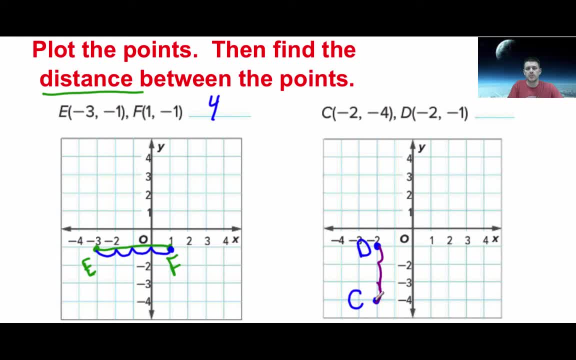 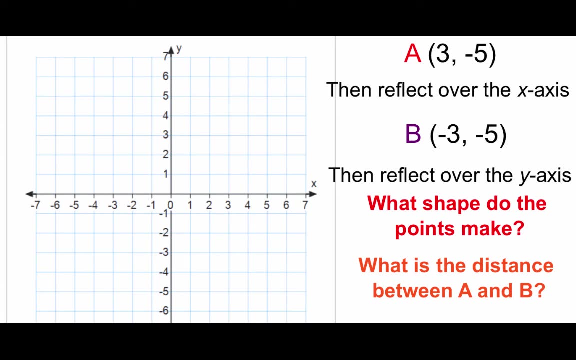 count the one you started on, but count one, two, three jumps to get to point C. So that's how we calculate distances. We simply plot the points and then see where did we go. Last one: if you needed to see a little bit more, If not remember, you can just watch whatever you need to of the video. 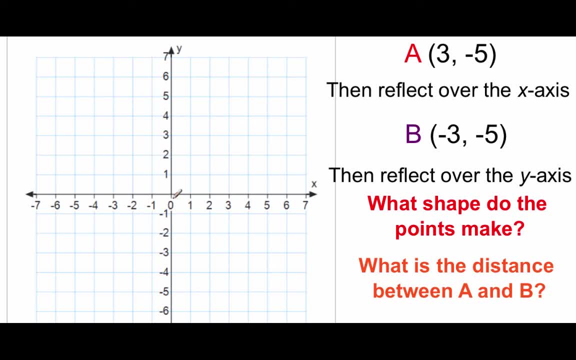 Point A is at three negative five. So first number is my X. So it means go over to three on the X and then go down to negative five on the Y, And it says reflected over the X axis. So here's my X axis, A little X that reminds you. So A is below the X axis, So I want to reflect above. I'm one. 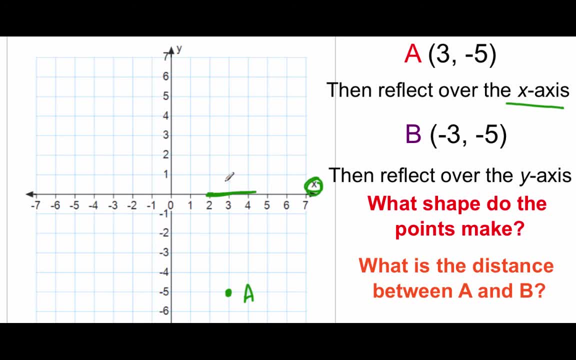 two, three, four, five units below. That's my new version A prime. Now point B is at negative three, negative five. So I always start at zero. I want to go left to negative three and then down to negative five. Remember the first. 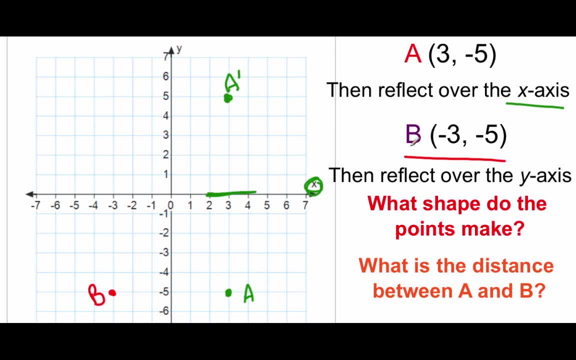 number is always your left and right. There's point B And I want to reflect over the Y axis, So Y, picture your mouth going wide open, And then point B is at negative three, negative five. So I always start at zero. I want to go left to negative three and then down to negative five. Remember the.